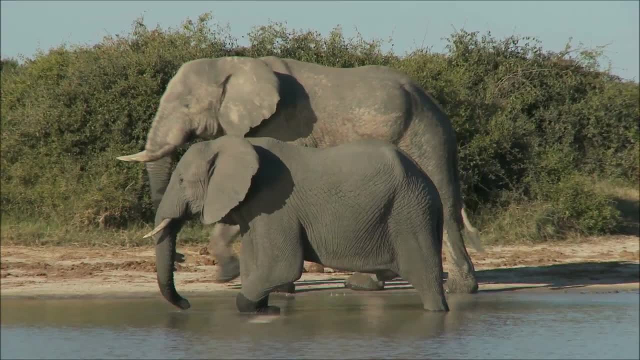 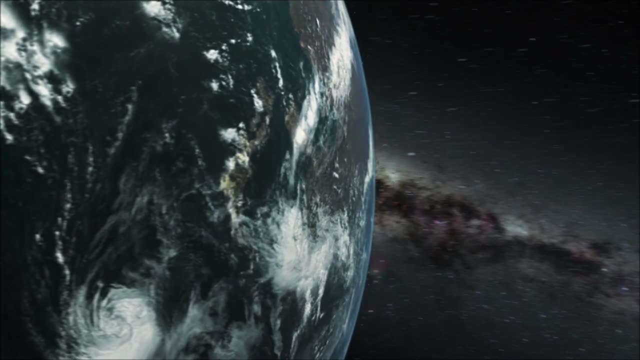 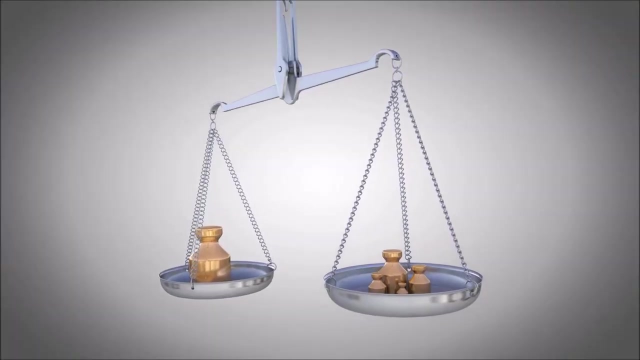 Of course you don't have very much gravity. The more mass something has, the more gravitational force it has. Compared to the gravity of the Earth, any gravitational force that you have is too weak to notice. Mass is not the same as weight. Mass is a measure of the matter. 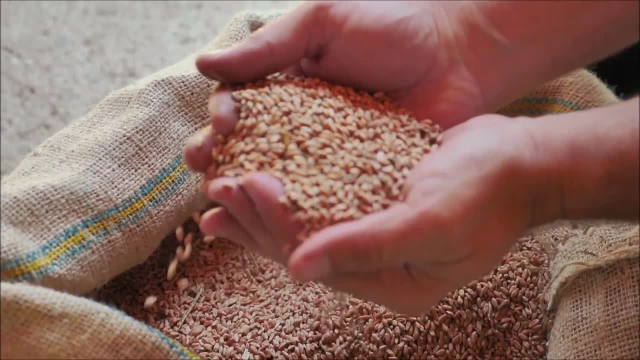 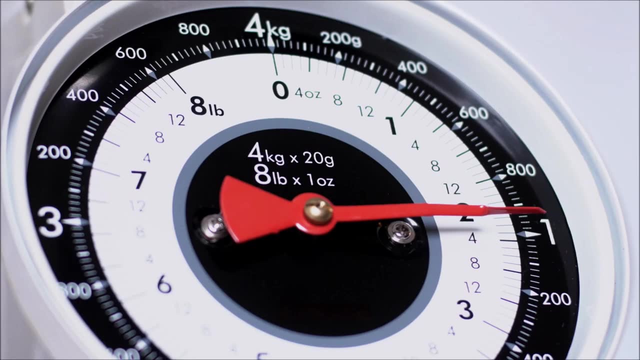 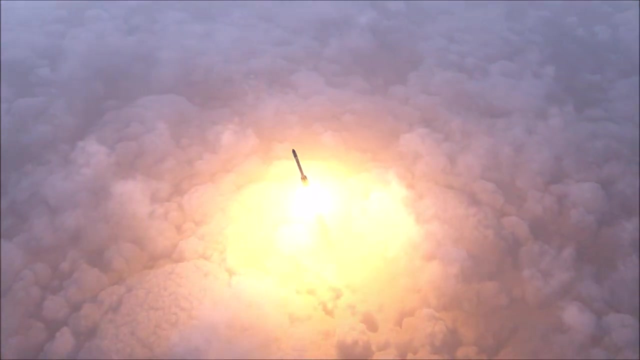 in an object and does not change no matter where you go. On the other hand, weight is a measure of gravity. Weight measures the pull of gravity on an object, and this can change. Most places on Earth have roughly the same amount of gravity, But if you were to leave Earth, the pull of 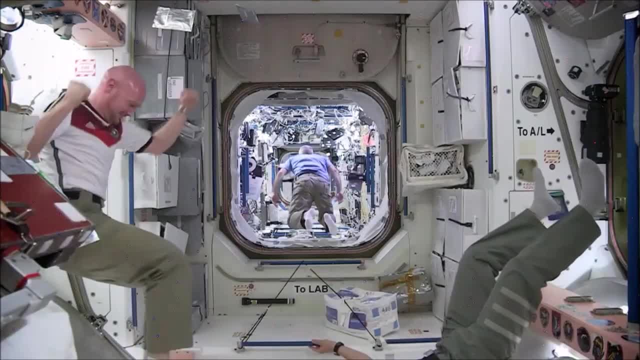 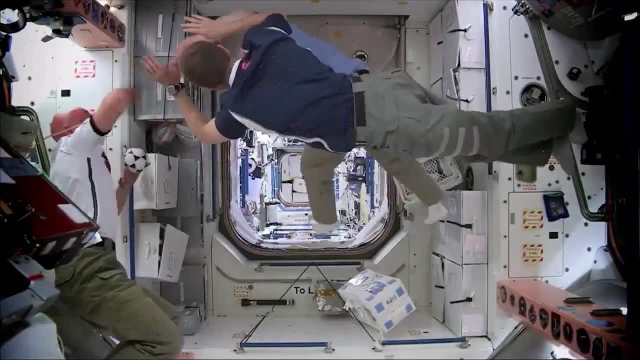 his gravity would weaken the farther away you went, until eventually you would experience zero g. This is because gravity gets weaker with distance. There is still gravity in space because everything that exists exerts this gravity force on its space. If you are so founded on gravity that you find that gravity can change If it does. 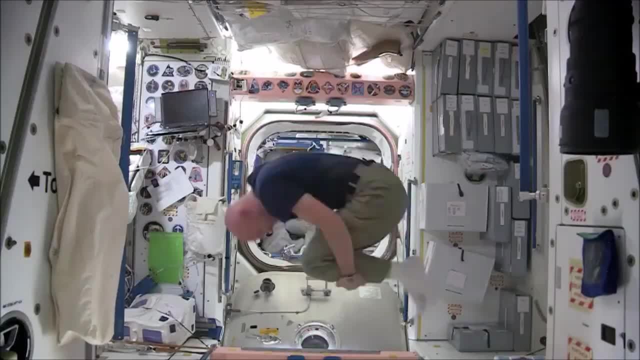 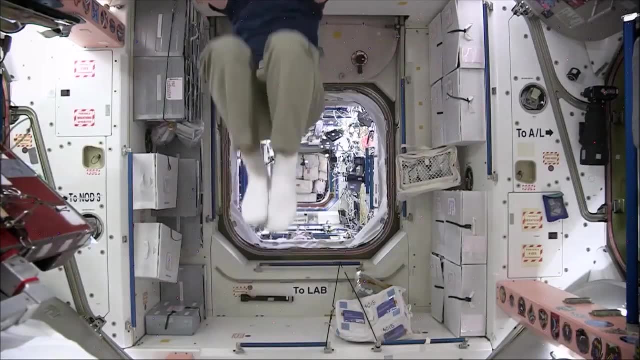 you can be filled with hope and be more howling, Like when you dropped a ball. But do you know something like this? Maybe there is gravitational force, But the gravitational pull from something like a person or even a spaceship is so small it feels as though you have no weight at all. 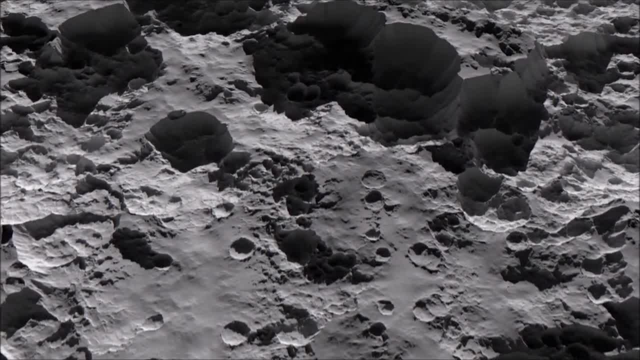 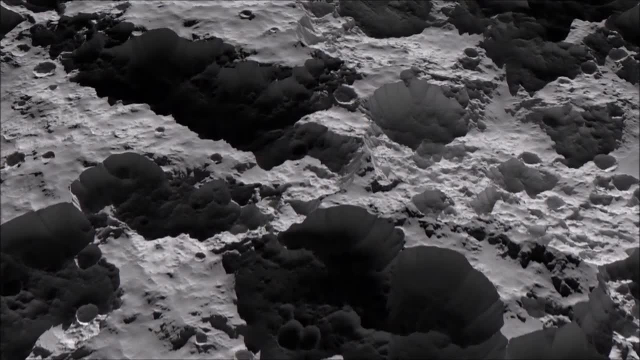 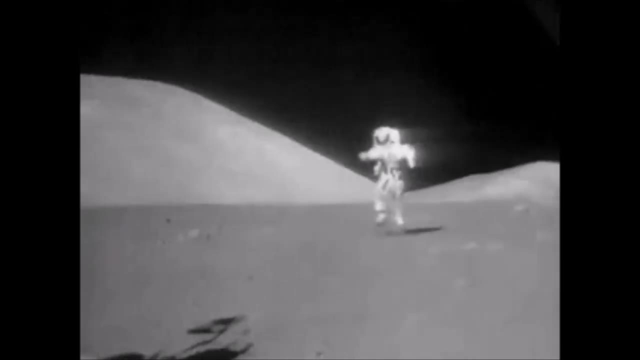 If you were to land on another planet or celestial body, the pull of gravity would be different depending on its mass, and you would not weigh the same as you did on Earth. On the Moon, for example, gravity is only about 17% of Earth's. This is because the 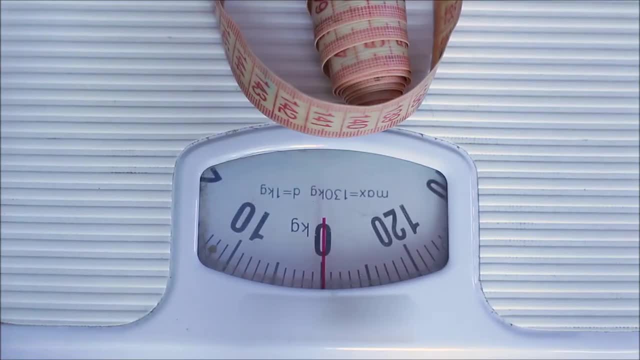 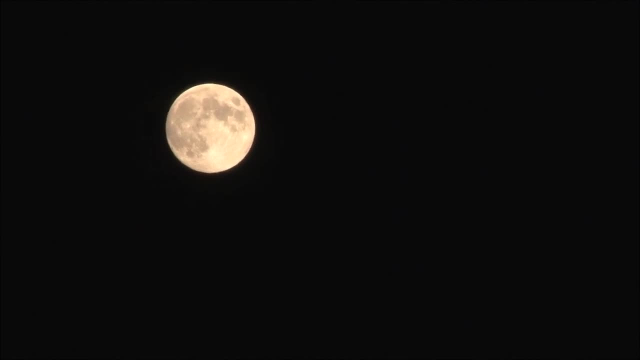 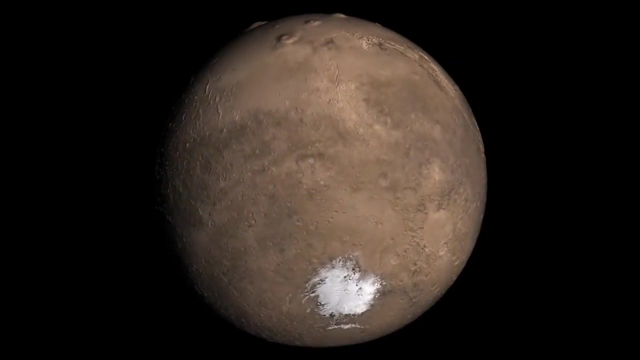 Moon is much less massive than the Earth. A person who weighs 100 pounds or 45 kilograms on Earth would weigh only 17 pounds or 7.5 kilograms on the Moon. On Mars, the same person would weigh 38 pounds or 17 kilograms. 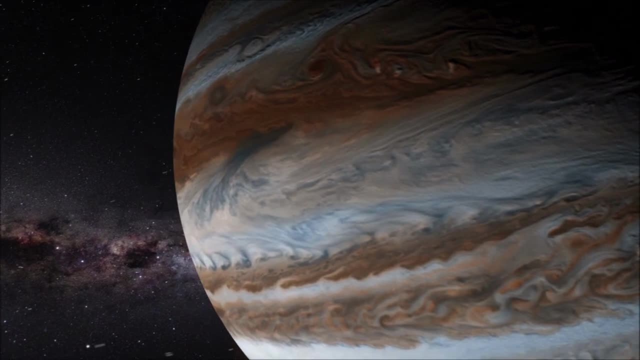 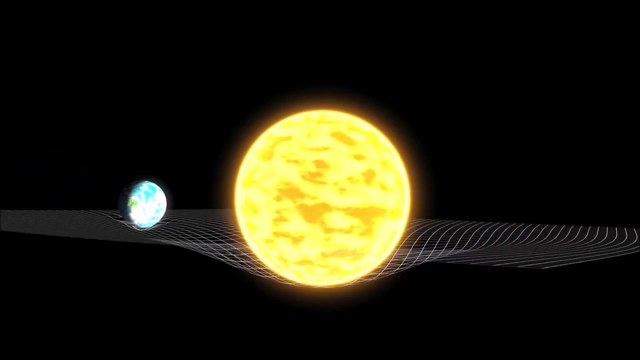 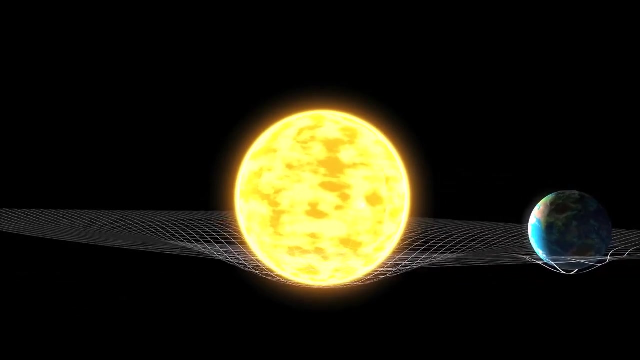 On Jupiter, they would weigh 253 pounds or 106 kilograms. Gravity is the weakest of the four fundamental forces of the universe and only gets weaker with distance, but it is very important for life on Earth. It is the force that holds us down to the surface of the planet.